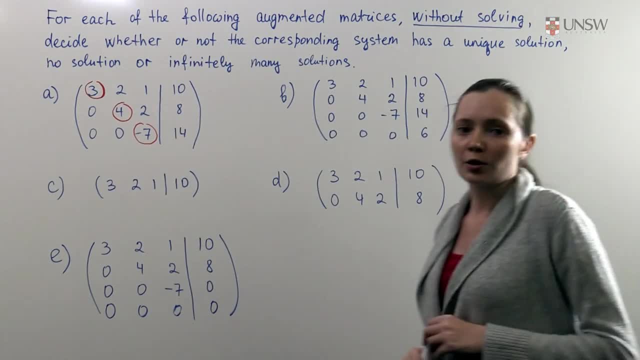 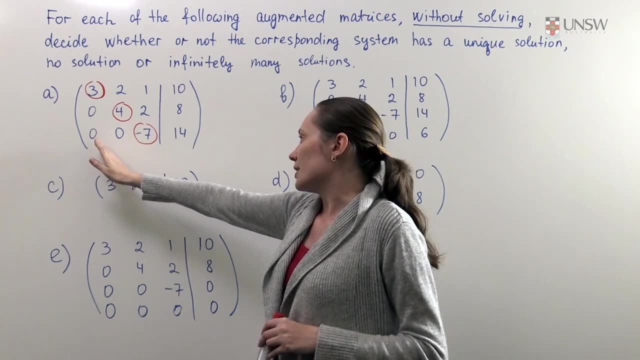 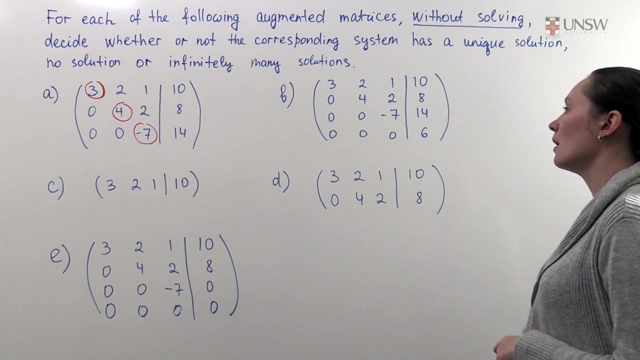 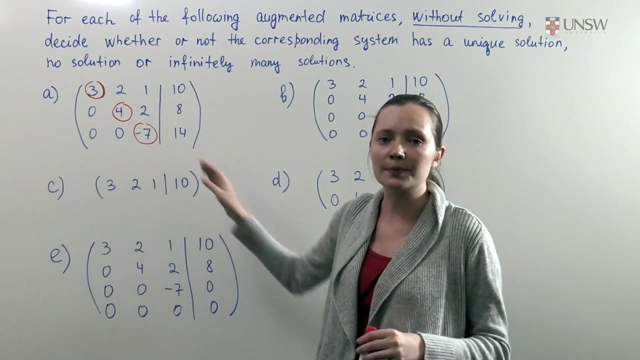 So this term is non-zero entry Columns are leading terms and the columns which contain leading terms we call leading columns. For example, these three columns are leading columns and this column is non-leading column. Okay, and the next step. we need to look at the constant vector. If the constant vector 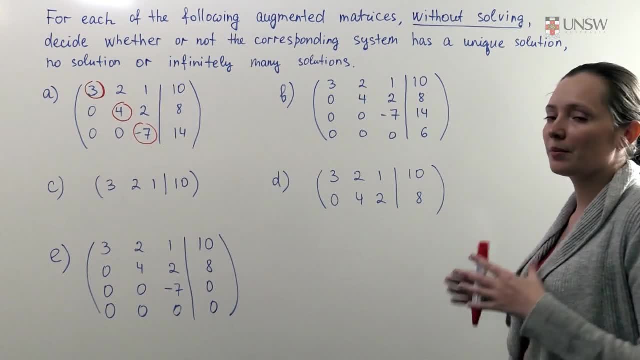 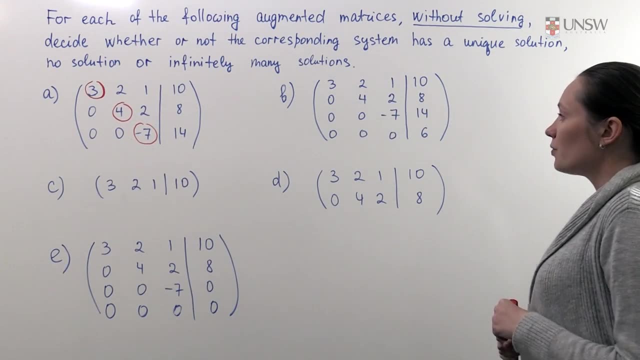 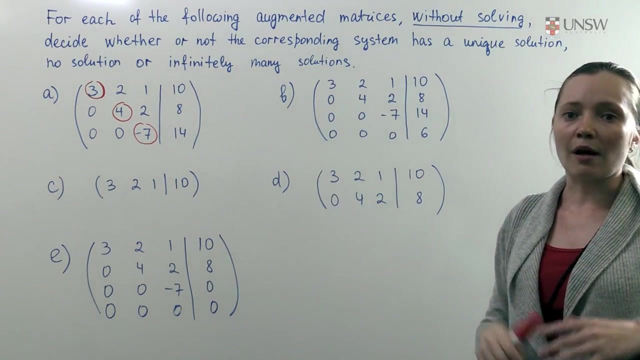 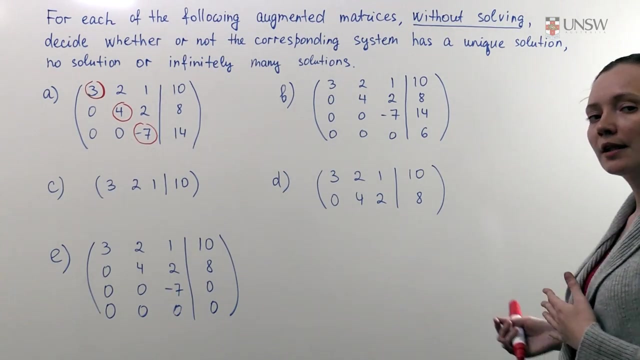 is a leading column, then the system has no leading column. In our case, the constant vector is non-leading column. Therefore we look at remaining columns, and if all remaining columns are leading columns, then the system has a unique solution. If at least one column is non-leading column, then the system has infinitely many solutions. 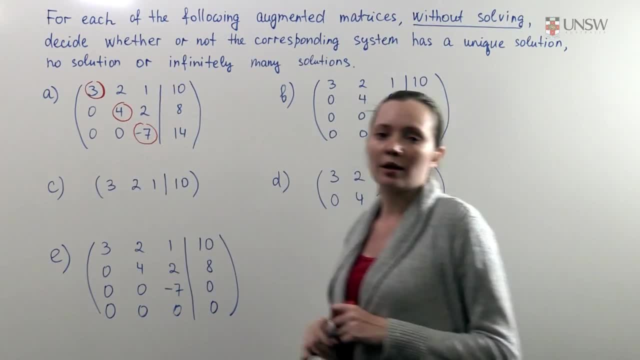 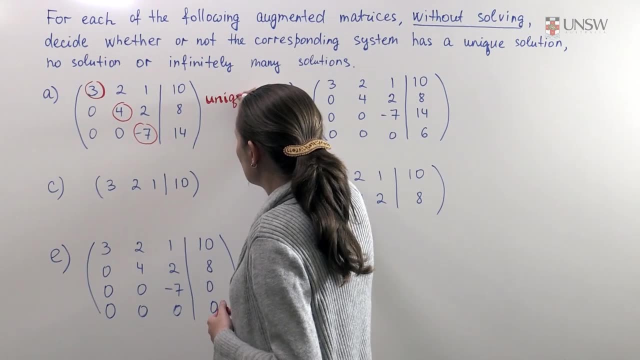 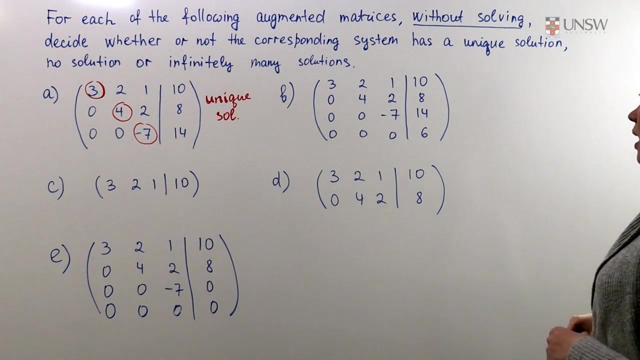 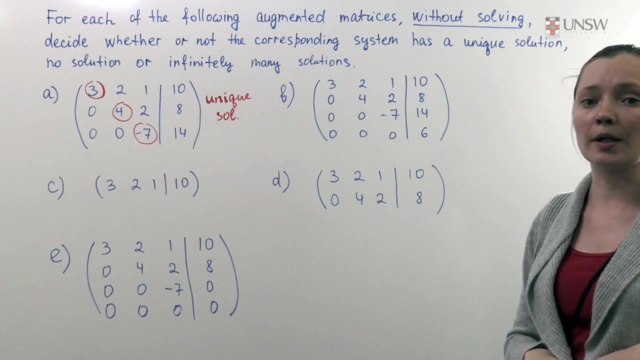 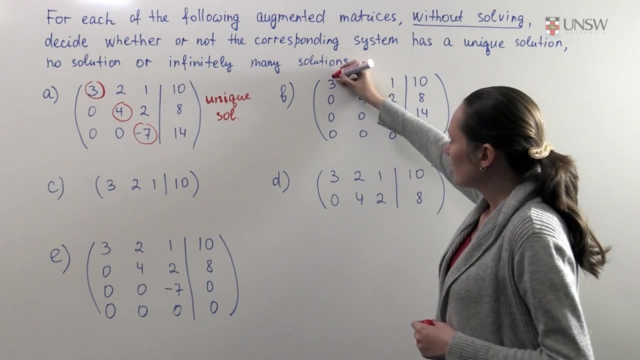 For example. in our case, all these three columns are leading columns. Therefore, we conclude that there is a unique solution for the corresponding system. Okay, let's do the matrix from part B Again. the first step is to determine all leading terms. We go along each row and as we meet the first non-zero entry, we determine the number of. 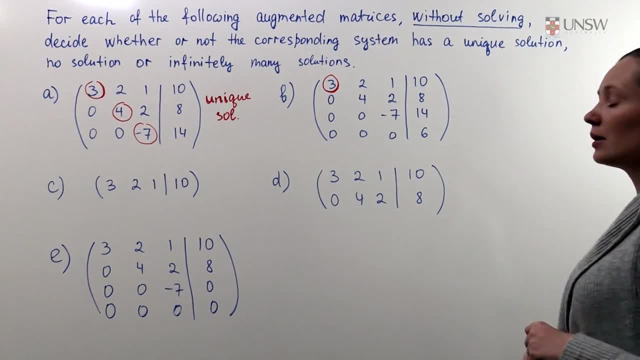 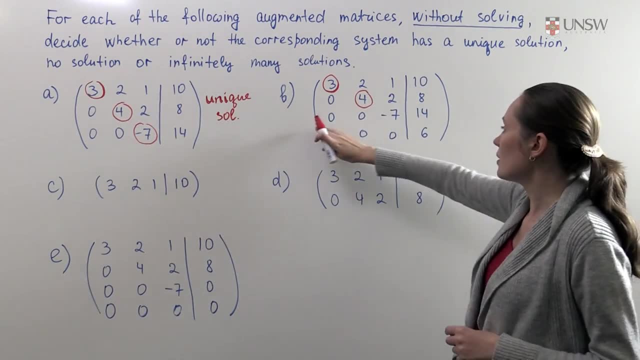 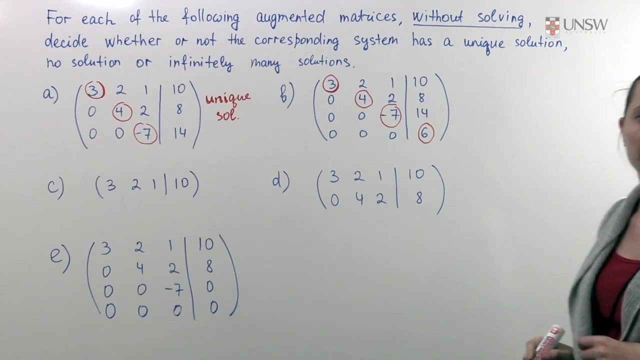 leading columns: the first non-zero entry, it will be leading term, okay. in the second row: this one is leading. in the third row: this one is leading. and fourth row: this one is leading. so in this case we have four leading columns. again, we look at the constant vector. 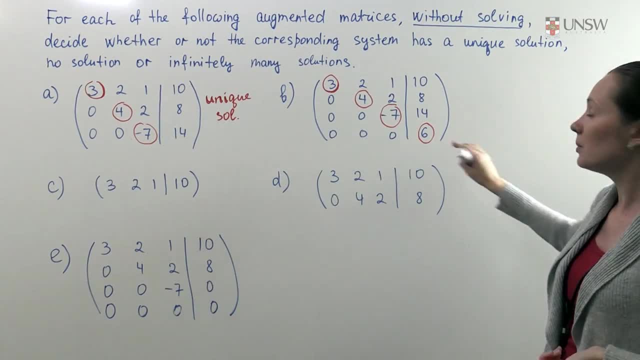 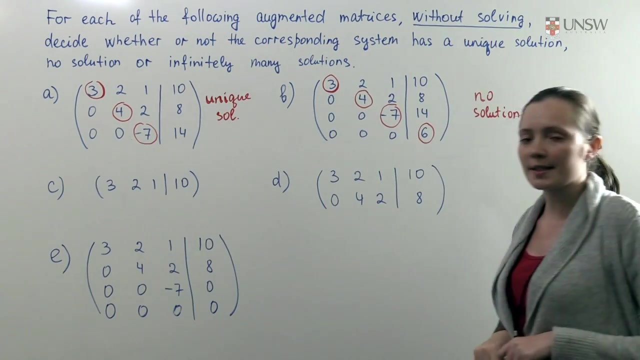 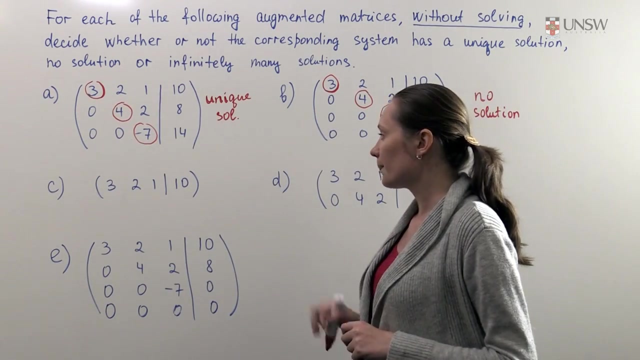 and in this case it's a leading column. therefore, we conclude that the system has no solution. okay, let's have a look at matrix from part c. then the same. firstly, we need to determine all leading terms and we have here only one reading term, so the first one is a leading term and the second one is a leading term.